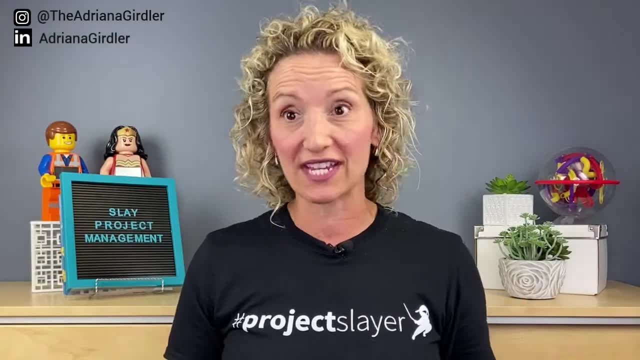 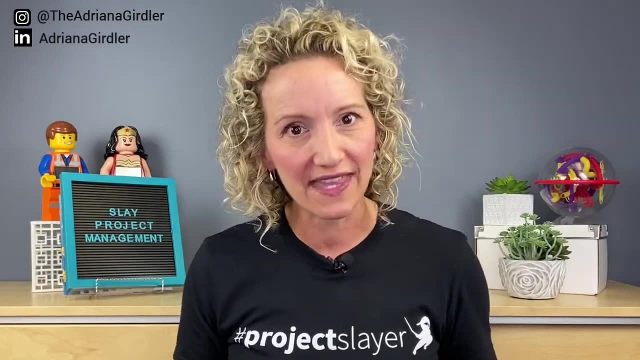 when I worked at an organization Amazing project. It was super intense And when it was over I was quite surprised with. I was actually sad that it was over, even though I was working 24: 7.. So that whole project closure is really important, but the celebration is really cool. 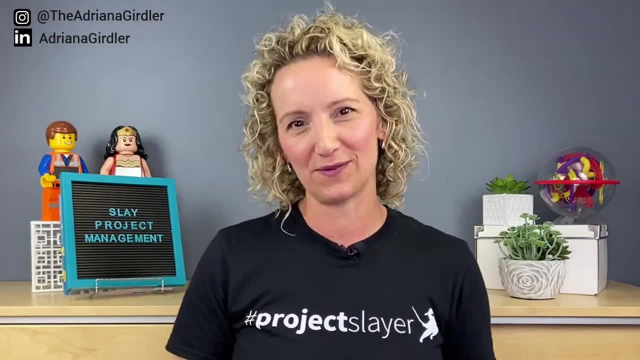 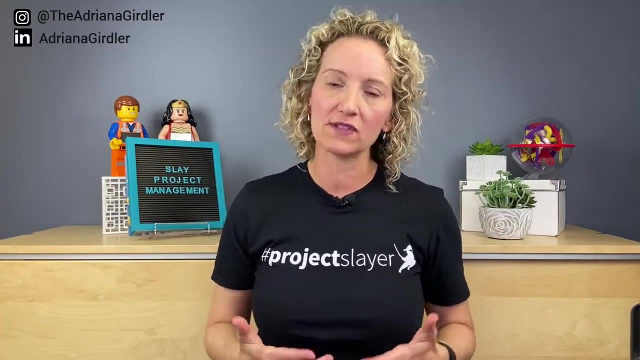 because it provides psychological closure to everyone who was involved. Conduct a project review Now. this is where you're going to do it with your team, And I call my project reviews after action reviews or AA reviews. I call them after action reviews or AA reviews. I call them. 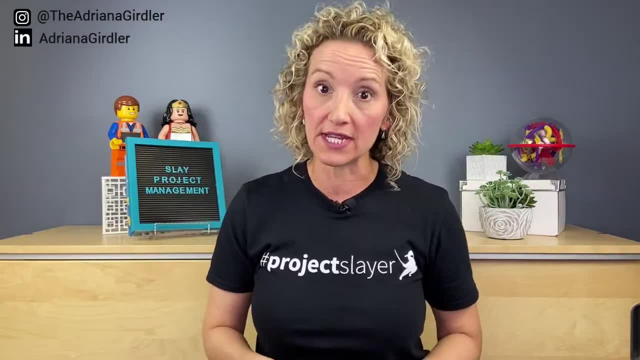 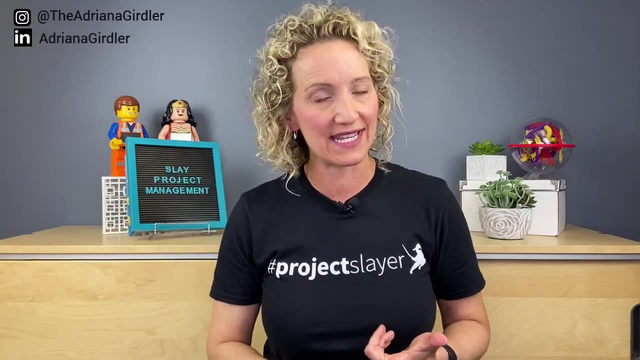 after action reviews or AA reviews. I call them after action reviews or AA reviews, And these are really important, because what you're really doing here is you're reviewing: how did it go with the project, What went well, What was planned, What came to fruition, What didn't. So these are all. 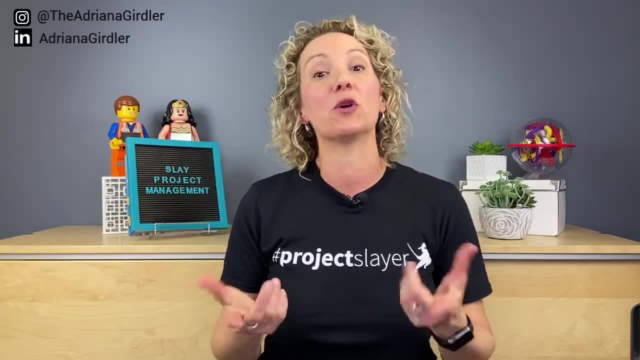 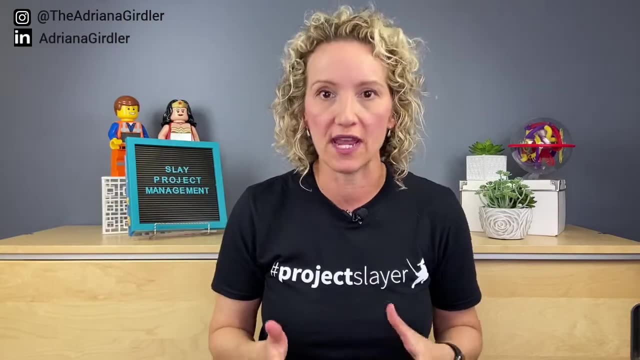 the key fundamentals that you're going to learn about your project. So did we do things on cost, time, budget, all of that stuff? Why do you want to do this? Because you don't want to reinvent the wheel. The whole purpose of an AAR and doing a review is to learn from it, get lessons learned. 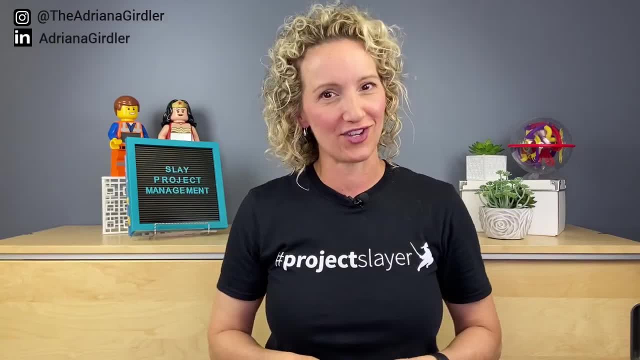 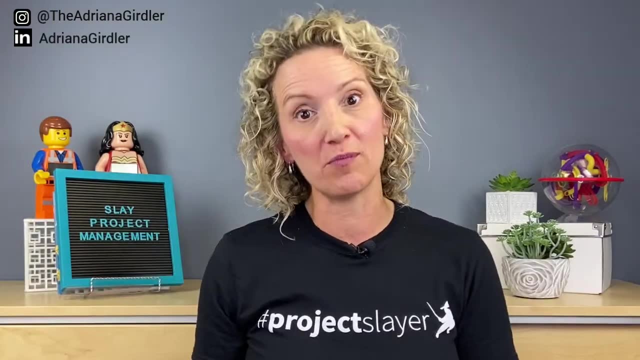 and to ensure you instill the power of AAR in your project, And that's what we're going to do. So, those lessons learned in your next project, Release resources and close out contracts. Okay, yes, I know we had a project celebration, but that didn't necessarily mean you officially. 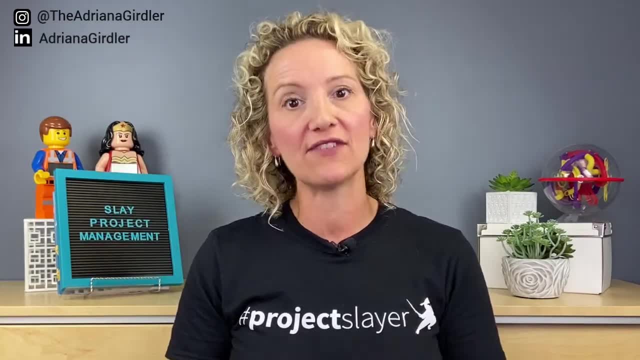 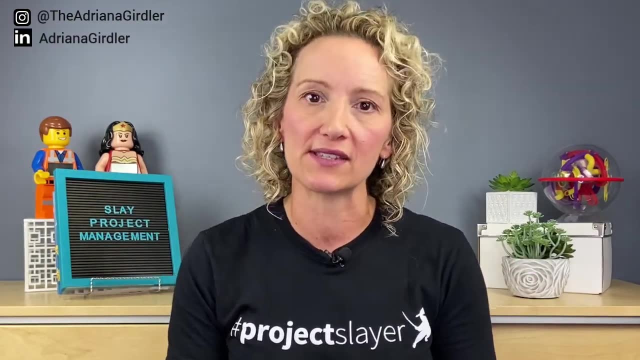 released people. You're going to have to take a look at your project. You're going to have to release the team, but you're going to have to keep a few people back, And what I mean by that is your project is not necessarily over just because you launched it. There's still a period of time of 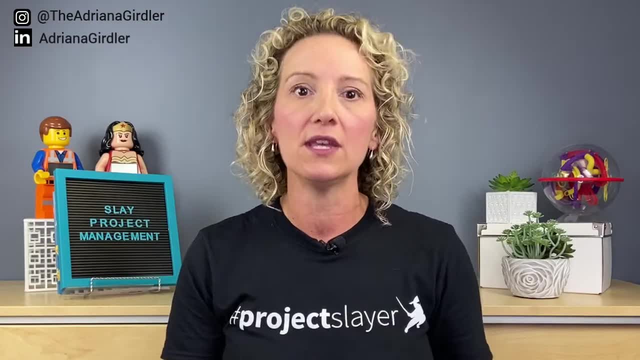 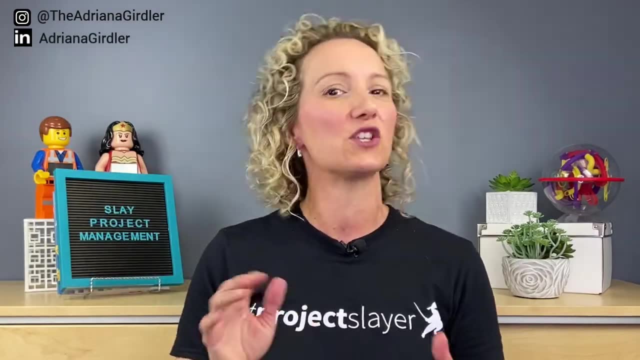 observation and you need a much smaller team in order to conduct that. So you have to make that official: Who's going to be staying on, who's not? You may even want to revamp a little bit of ways of working, because it is a little bit different when you're kind of overseeing and 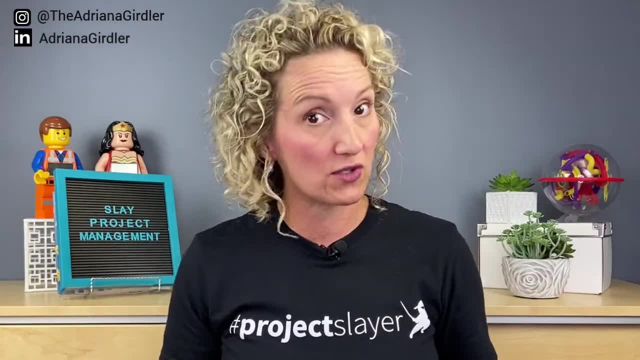 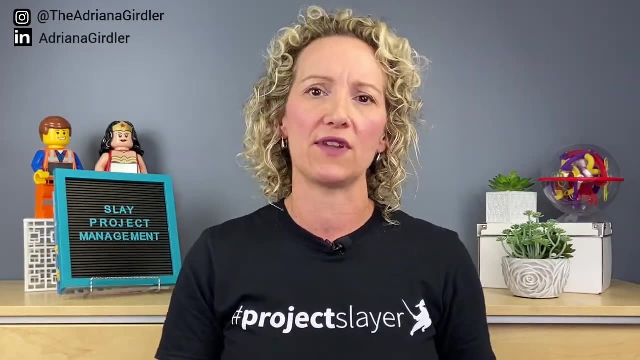 observing what it is that you implemented. Now you're also going to have to close out all contracts. You may have had some suppliers that were helping you on and you want to make sure that they're paid. You want to make sure that everything is signed off and that you are. 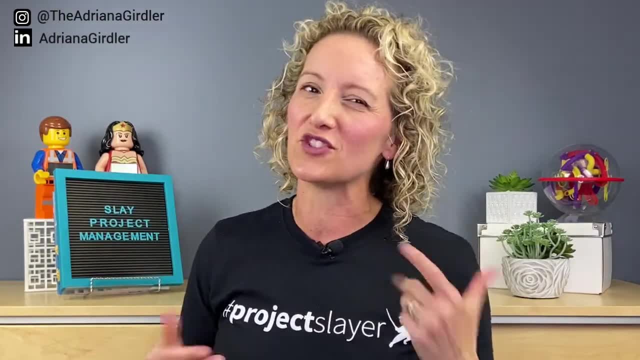 happy with the work that they've done as well, But I'm assuming you are, because you would have checked with them throughout the whole life cycle of the project. But again, this is really, really important from a closing out of a project. So that's what we're going to do today.